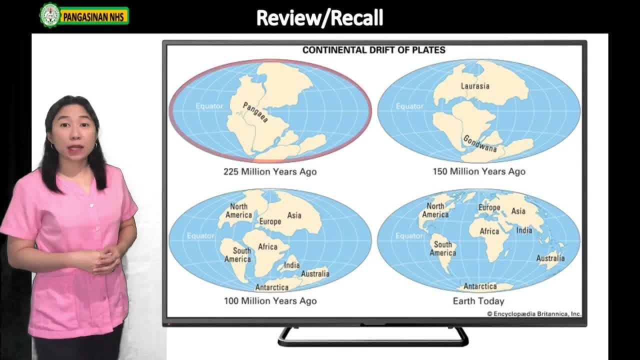 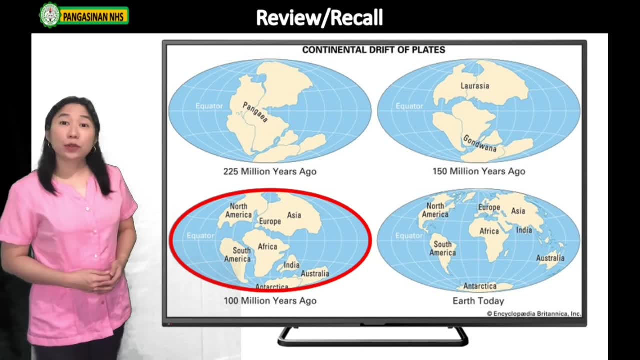 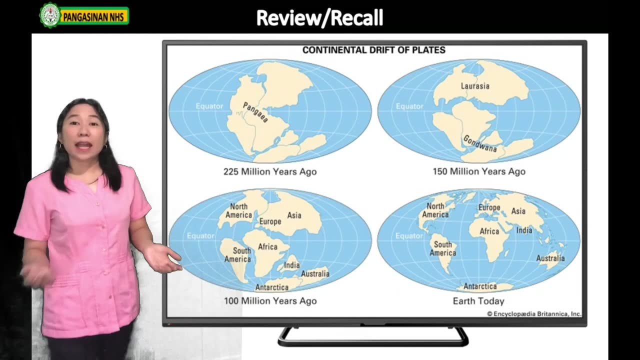 This supercontinent, Pangea, was divided into two supercontinents named Lauritia and Gondwanalan. Pieces of Lauritia drifted to the north, while pieces of Gondwanalan drifted to the south And eventually drifted into day 7 continents. 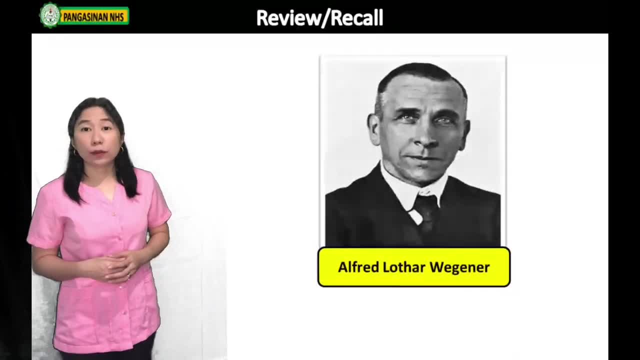 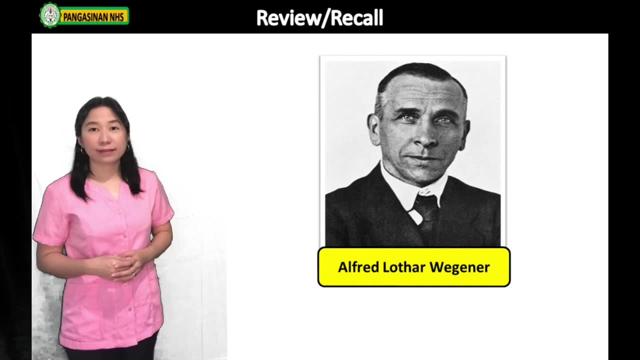 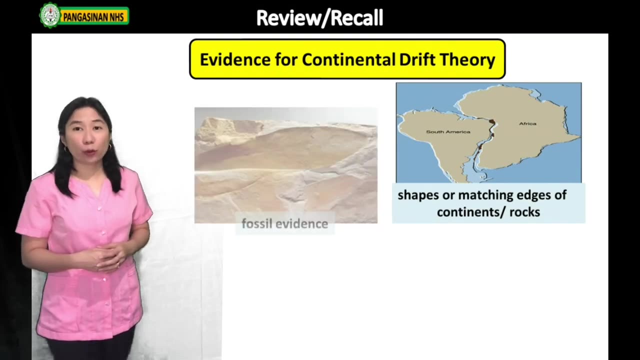 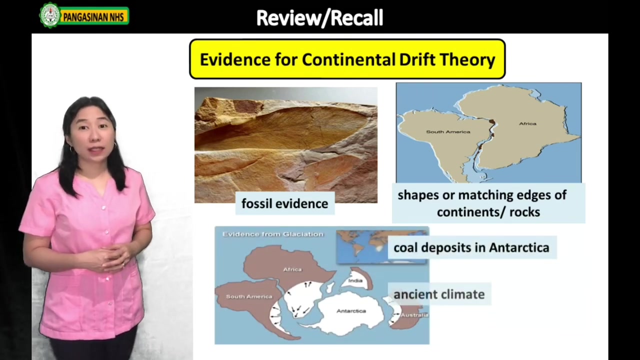 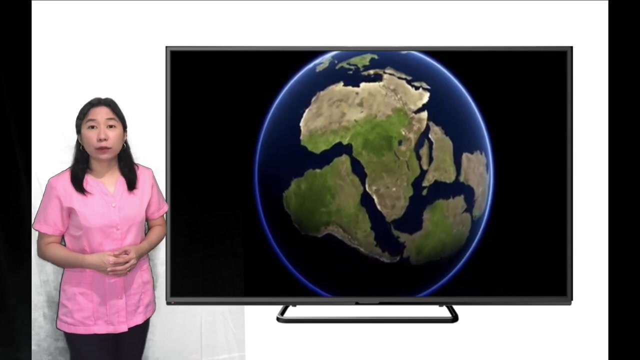 Alfred Wegener, the originator of the Continental Drift Theory, identified several evidence to support his claim that continents are drifting around the Earth. These evidence are. Despite of these evidence, the Continental Drift Theory was still rejected during Wegener's time because he can't explain what causing the continents to drift. 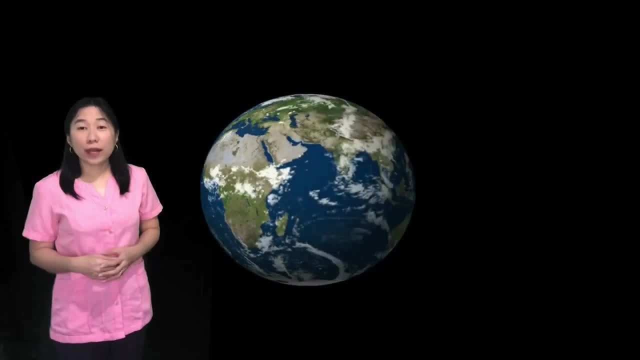 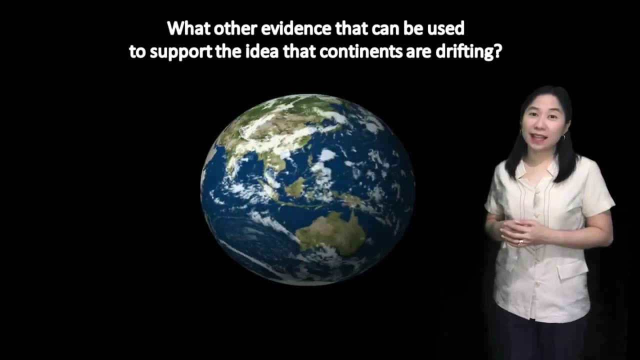 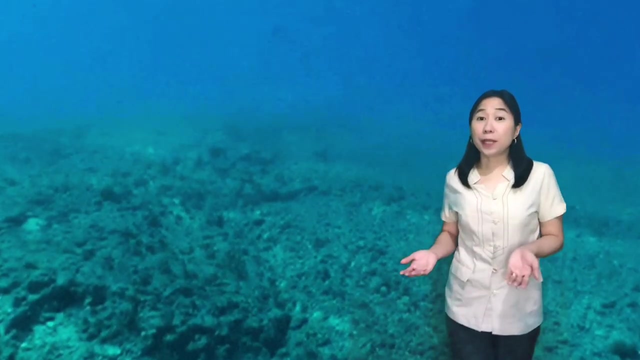 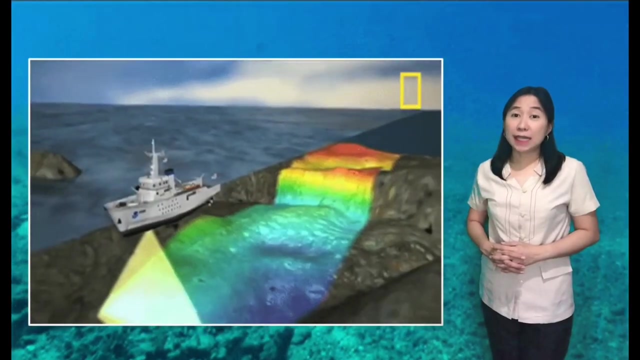 What other evidence can be used to support the idea that continents are drifting? Let's find out in today's lesson. Seafloor Spreading. Many people in the past believed that the ocean floor is flat like the desert. But in 1930s, where sounding geared, cold sonar was developed, 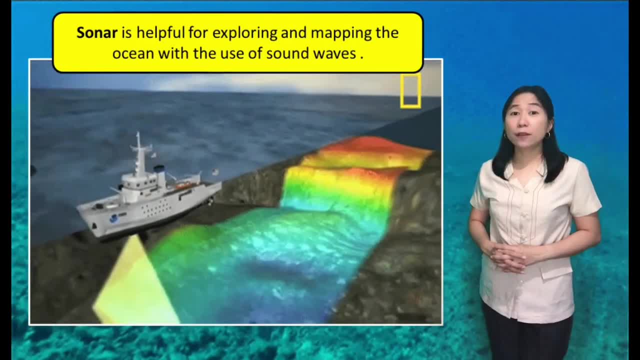 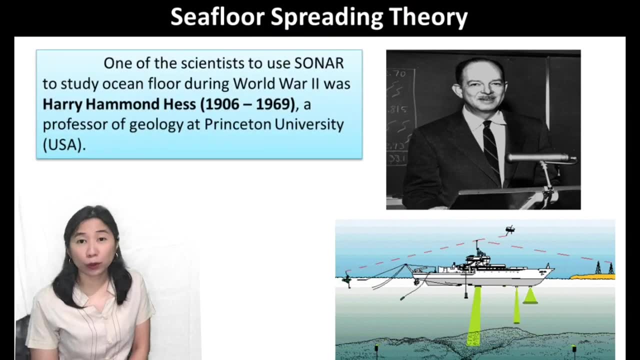 it was called a seafloor. It leads to the discovery of the standing feature of the ocean floor. One of the scientists to use sonar to study ocean floor during World War II was Harry Hammond Hess, a professor of geology at Princeton University. 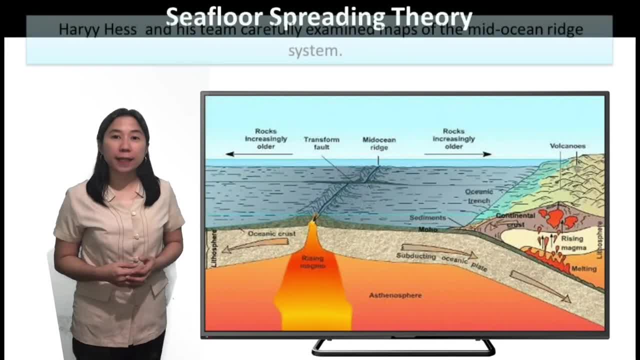 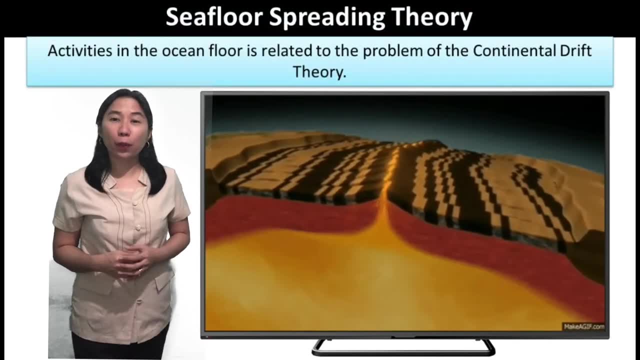 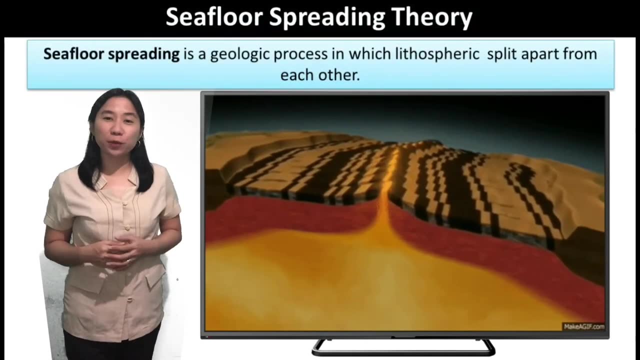 Harry Hess and his team carefully examined maps of the mid-ocean ridge system. Then Hess began to think about the ocean floor in relation to the problem of the Continental Drift Theory. That leads him to the idea of seafloor spreading. According to the seafloor spreading theory, 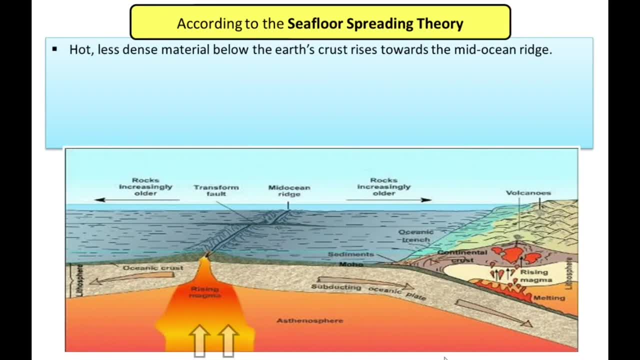 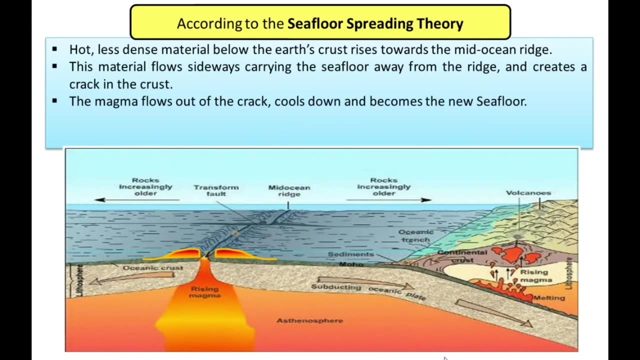 hot, less dense material below the Earth's crust rises towards the mid-ocean ridge. This material flows sideways, carrying the seafloor away from the ridge, and creates a crack in the crust. The magma flows out of the crack, cools down and becomes the new seafloor. 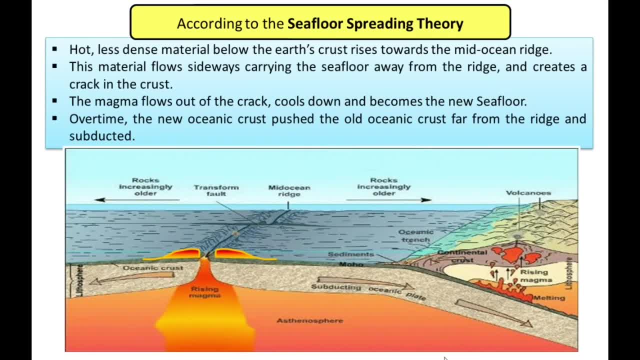 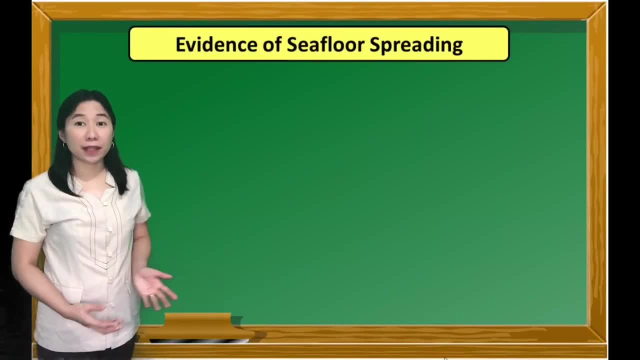 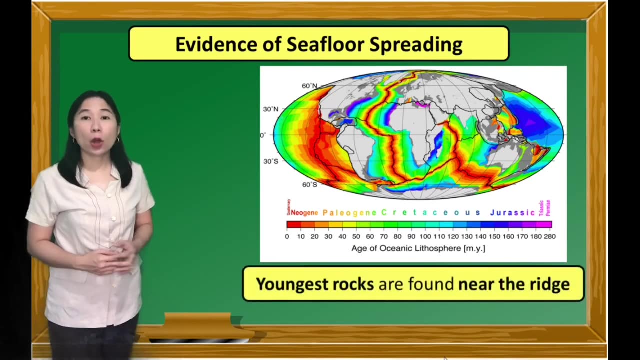 Over time, the new oceanic crust pushed the old oceanic crust far from the ridge and subducted. The idea of seafloor spreading is supported by this evidence. Scientists find out that youngest rocks are found near the ridge, while oldest rocks are found far from the ridge. 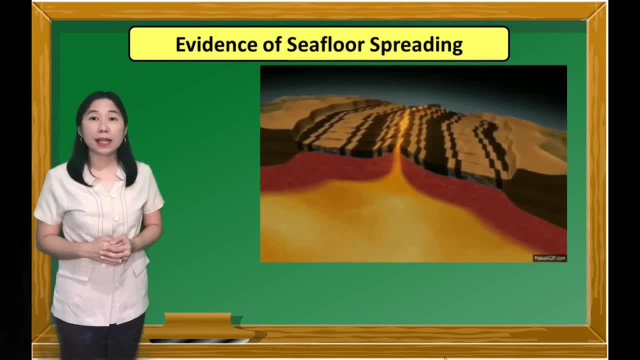 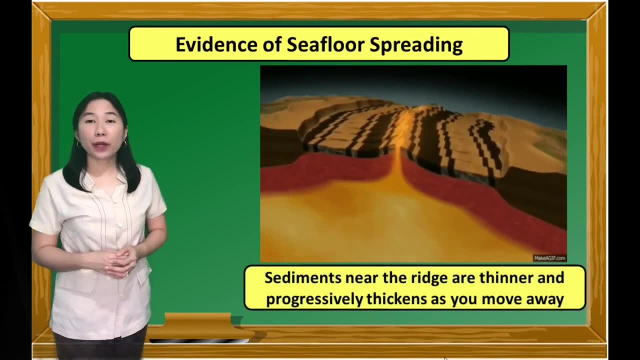 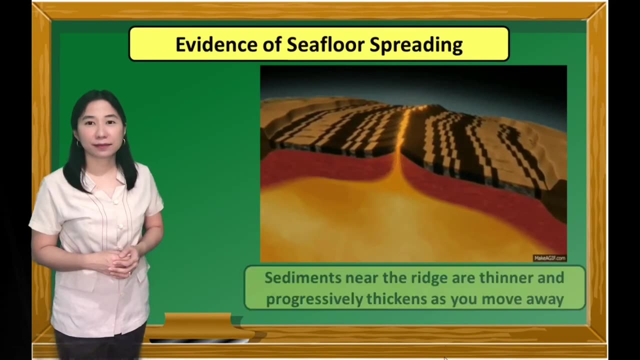 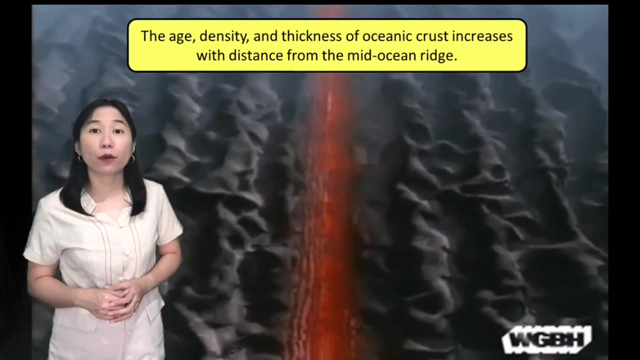 This provides evidence that seafloor spreading and new crust is being created at the ridge. Since there's spreading happening at the ridge, the sediments near the ridge are thinner and progressively thickens as you move away. Always remember that the ages, density and thickness of the oceanic crust increases with distance from the mid-ocean ridge. 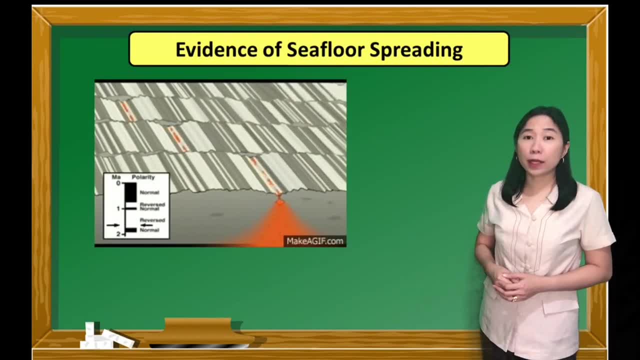 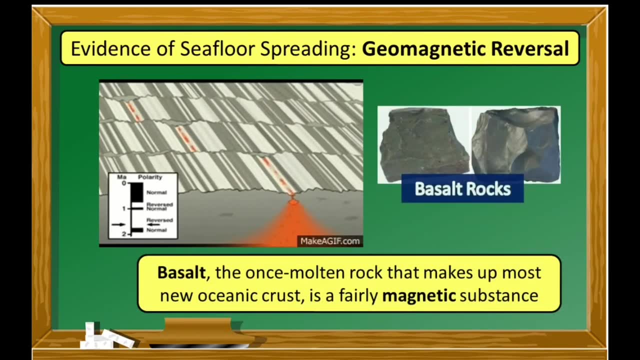 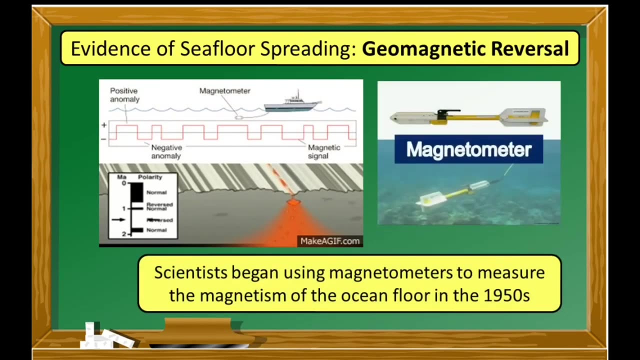 Another strong evidence that supports seafloor spreading is the geomagnetic reversal Basalt, the once molten rock that makes up most new oceanic crust, is a fairly magnetic substance. Scientists began using magnetometers to measure the magnetism of the ocean floor in the 1950s. 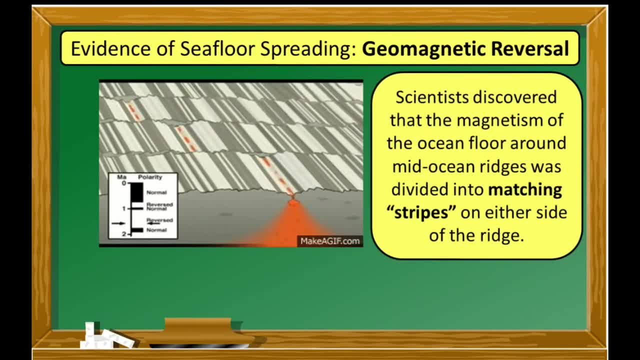 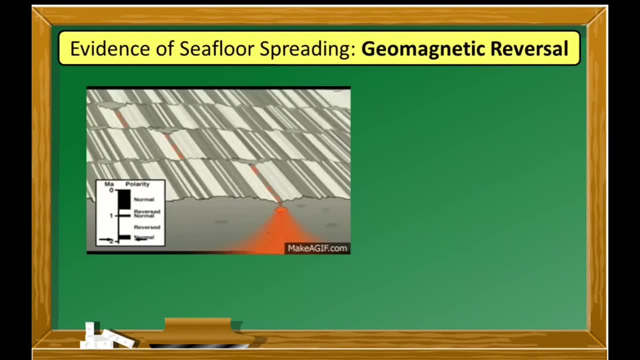 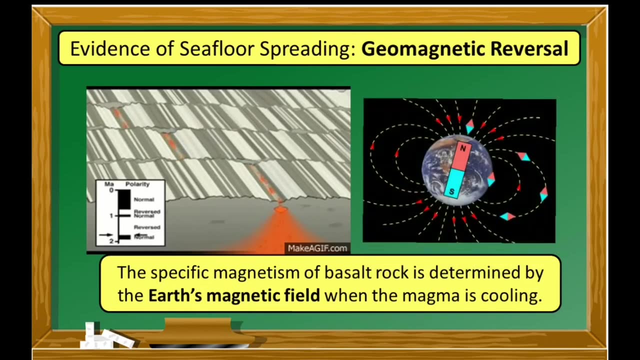 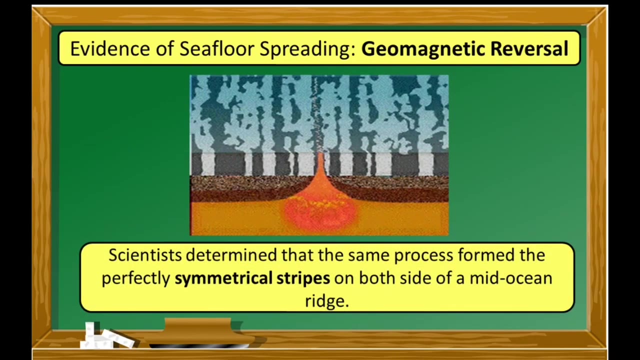 Scientists discovered that the magnetism of the ocean floor around mid-ocean ridges was divided into matching stripes on either side of the ridge. The specific magnetism of basalt rock is determined by the Earth's magnetic field when the magma is cooling. Scientists determined that the same process formed the perfectly symmetrical stripes on both sides of a mid-ocean ridge. 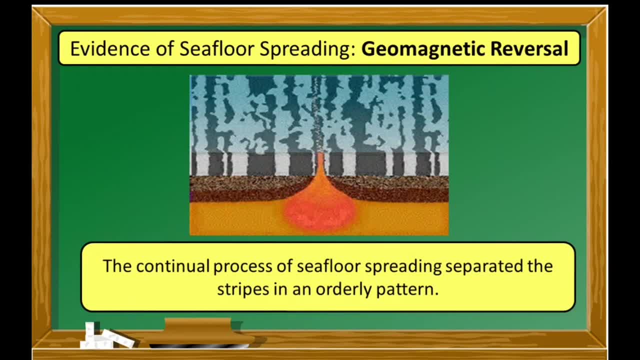 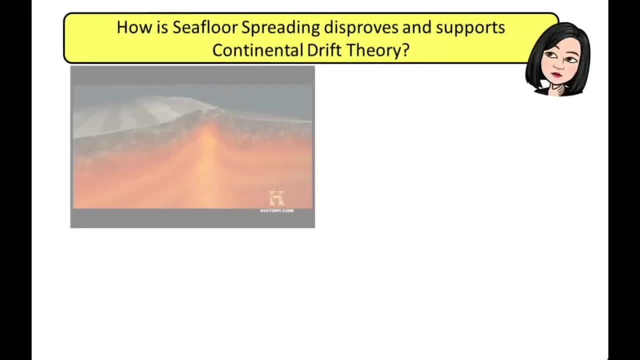 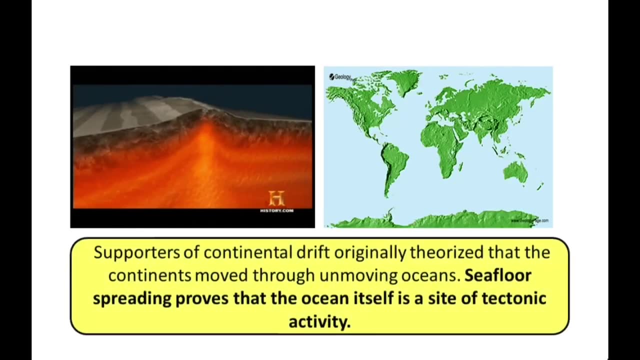 The continual process of seafloor spreading separated the stripes in an orderly pattern. How is seafloor spreading? disproves and supports continental drift theory. How is seafloor spreading? disproves and supports continental drift theory. How is seafloor spreading? disproves and supports continental drift theory. 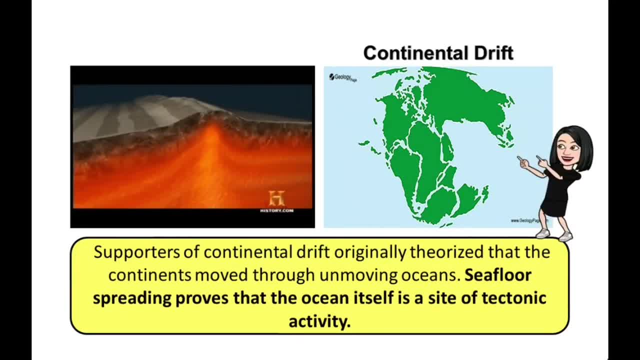 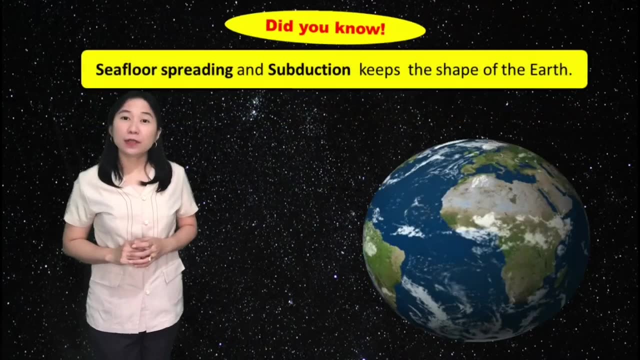 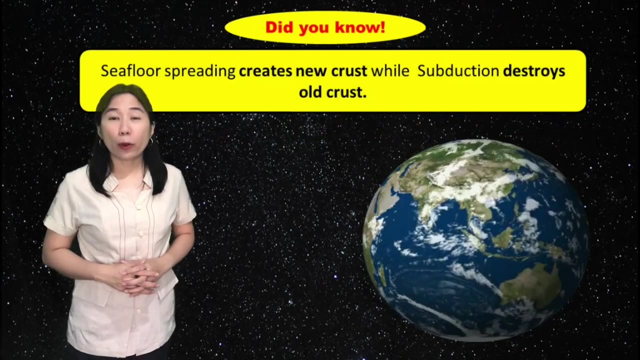 reef originally theorized that the continents move through unmoving oceans. seafloor spreading proves that the ocean itself is a site of tectonic activity. did you know that seafloor spreading and subduction keeps the shape of the earth? seafloor spreading creates new crust, while subduction destroys old crust. the